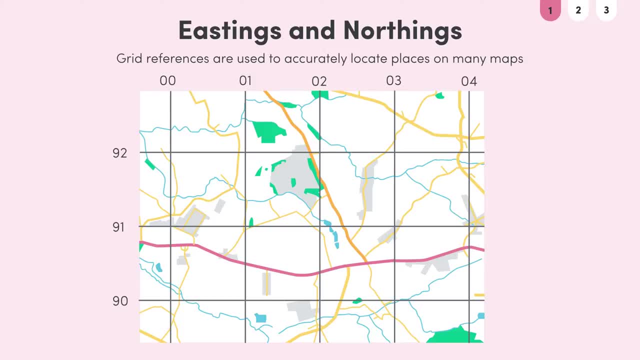 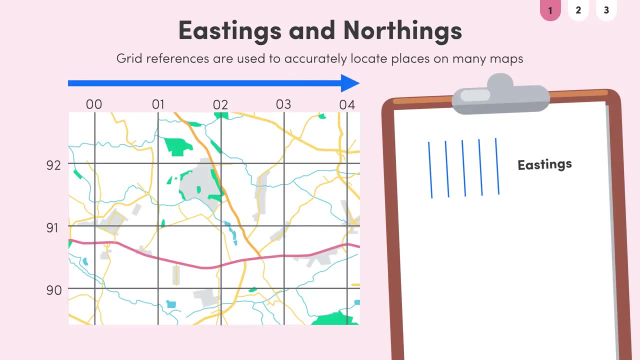 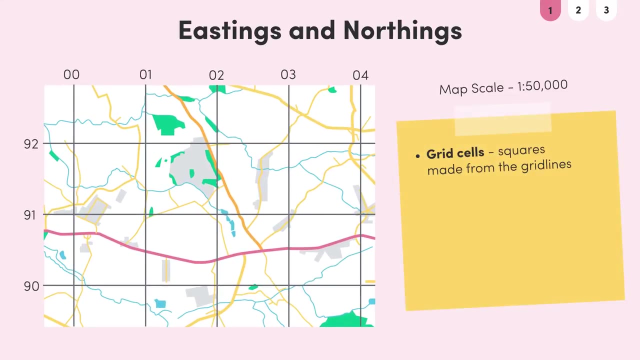 numbered lines. These numbers are used to identify the lines. The vertical lines are called Eastings, as their numbers increase towards the east. The horizontal lines are called Northings, as their numbers increase towards the north. These grid lines make squares, called grid cells, which can be identified using four-figure. 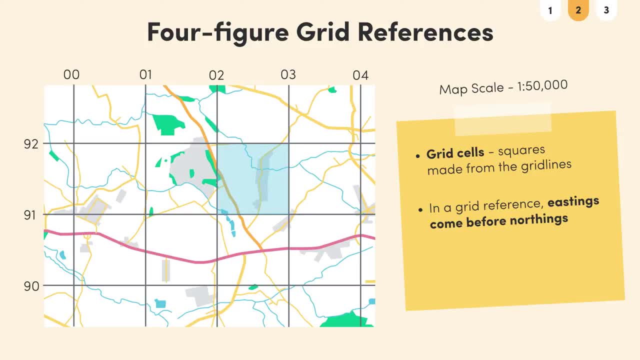 grid references. When giving any grid reference, the Eastings are given first, followed by the Northings. In the case of a four-figure grid reference, the point on the bottom left of the grid cell is used to find the reference. For example, in this map, with a scale of one, 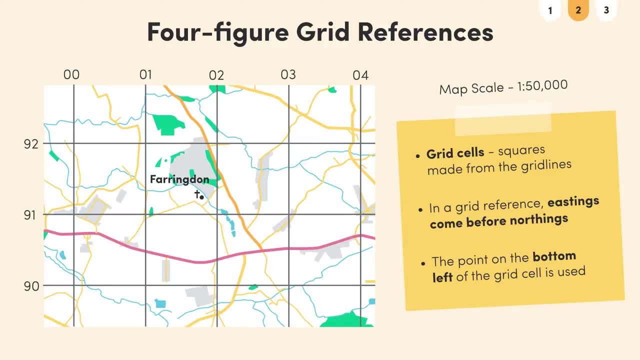 to fifty thousand. the church in Farringdon lies in this box. here To find the four-figure grid reference, we can see that the bottom left corner of the square lies on the Easting 01 and the Northing 91. So if we put these together we find that its grid reference is 0191.. 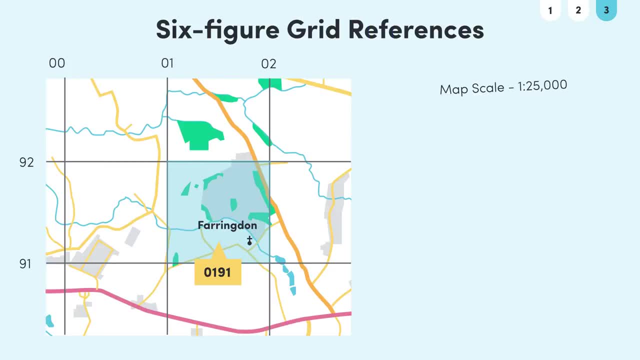 Sometimes, though, four-figure grid references aren't precise enough. This is especially the case for maps with larger scales. This means that the grid cells are larger to show more information, so you need to be more precise to be able to exactly locate particular features. For example, if we take a larger scale view of the same area of Farringdon from the last 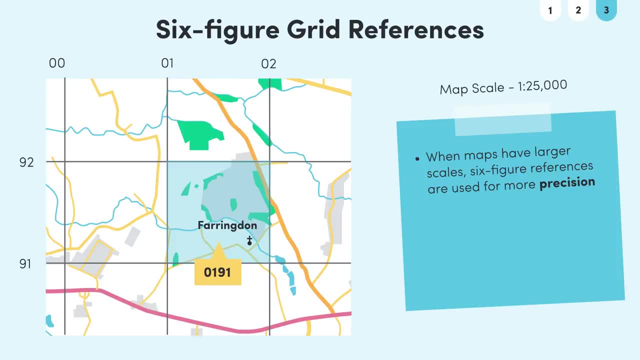 example, but now at a one to twenty five thousand scale, we can see that the grid cell is a bit too big to provide a precise location of the church. So the way we figure out a 6-figure grid reference is to mentally divide our cell of interest. 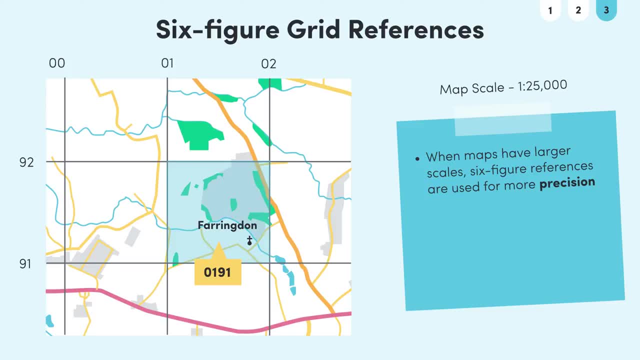 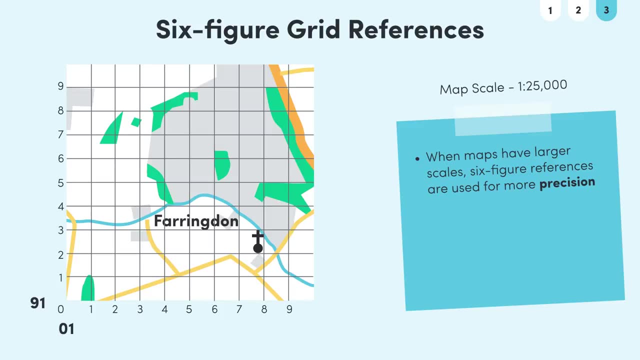 so, in this case, the cell defined by the 4-figure grid reference 0191, into a 10x10 grid. If we use our imagination to zoom in on the cell, we will eventually get the same result, but this is what we can see. When finding a six-figure grid reference, we're looking for the closest. 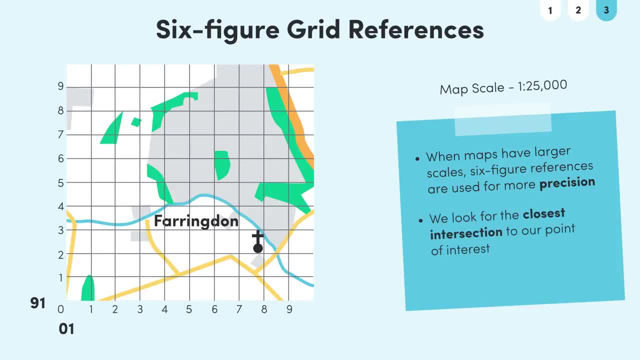 intersection of these smaller grid lines to our point of interest. In this case the church is found closest to this point. here The closest easting reference is eight squares along O1 and the closest northing is two small squares up from 9-1.. So the six-figure grid reference.